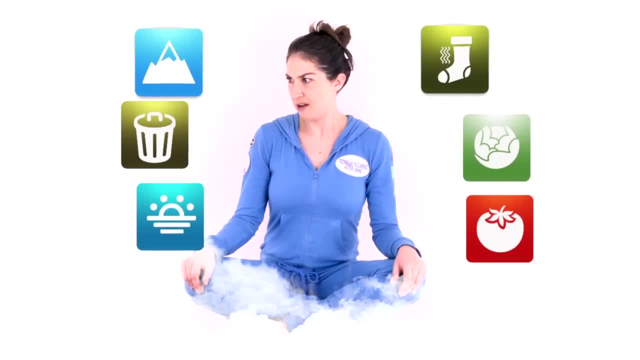 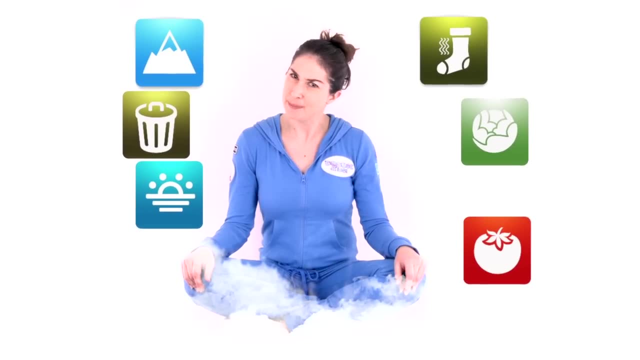 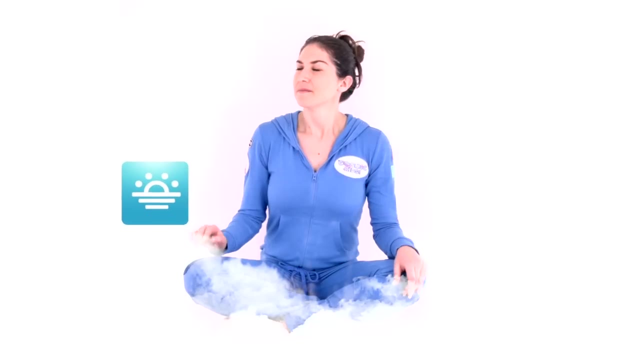 What have we got here? The smell of garbage in the bin. Not really A tomato smell, Maybe not right now. Here's one. Yes, let's smell the sea. Ahhh, yes, that is a fresh, salty and clean smell. now we get ready to go on a. 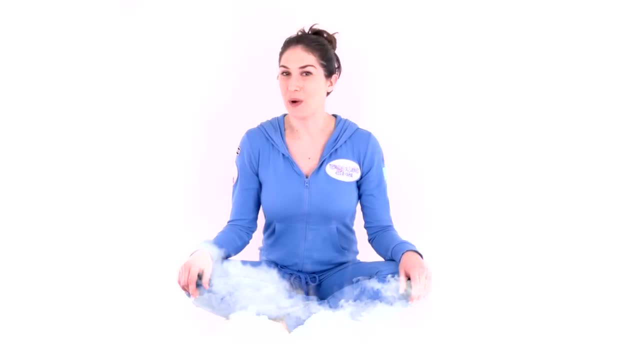 special journey. We're taking a trip on a boat, A boat in our minds, which means we can make this boat just how we like it. So close your eyes and find your boat in your mind. It might take a moment to appear, but it is dark when we 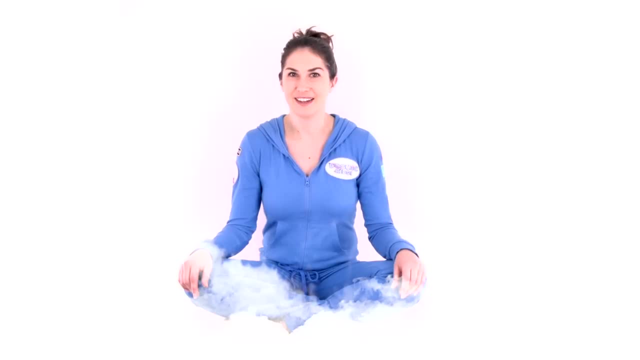 first close our eyes. Now we can see. we're at the beach and our boat is there where the ocean waves lap the sand of the shore. It's bobbing up and down lightly as the water moves. Now let's find out a bit more about your boat. What? 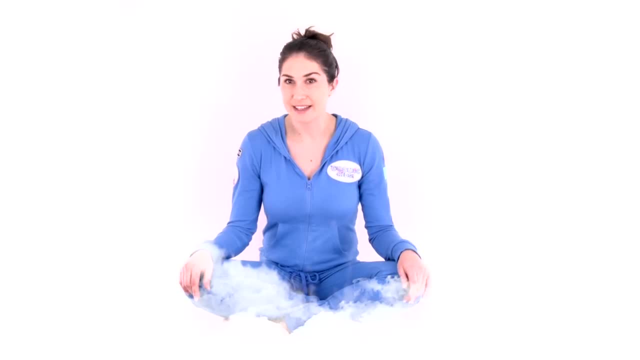 colour is it? Does it have a sail? We go closer to have a look inside. Wow, is that your big, comfy seat inside? Gosh, it's big enough for you to lie down in. That's cool. It looks like a lovely boat. You're ready to head out and spend some time in your 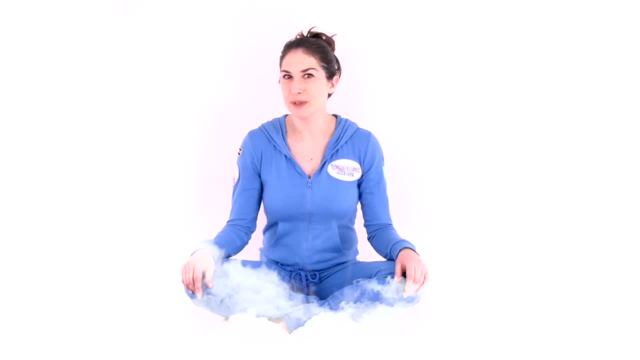 boat. So you hop in and with a little push you're off, Being carried by the waves out to sea. You can still hear me and enjoy this special time to lie back on your big comfy seat. Ah, that's a nice feeling. The. 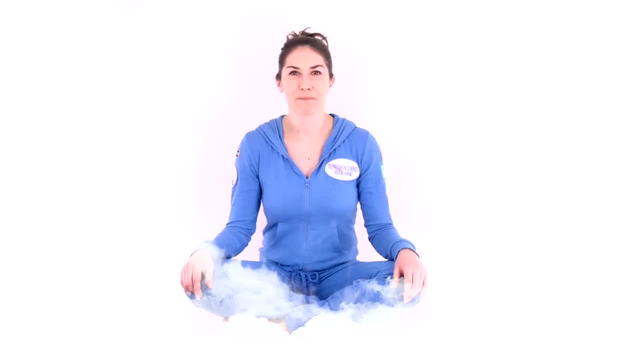 sun feels warm on your face and body. The ocean waves gently rock you in the boat. It's very peaceful here out at sea. You can hear the waves and the waves and the sound of the birds above and far away, Little splash, sounds of water as the 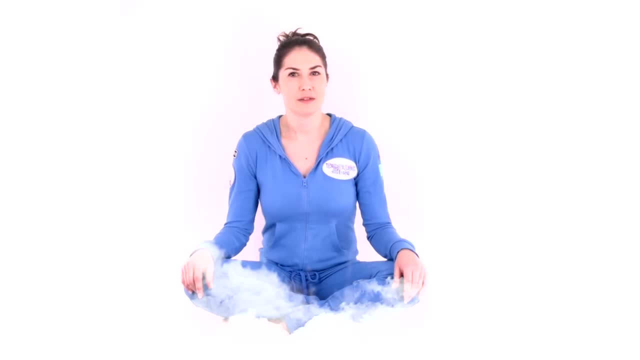 waves meet the boat. Now you hear another sound humming. It's very quiet in the distance, but it starts becoming louder and clearer as it comes nearer to you. You recognise the sound as that of another boat. Its engine is making the humming sound. 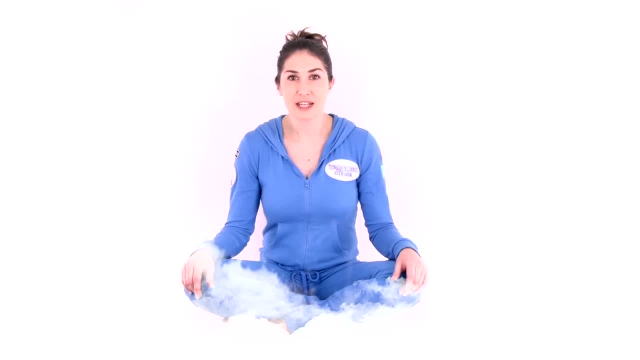 It's close now and it slows down as it reaches your boat. You see the driver is a kind old man. He's smiling peacefully. He pulls up next to your boat, turns the engine off and tells you he has brought the bye-bye boat for you. He then asks for your worries. He 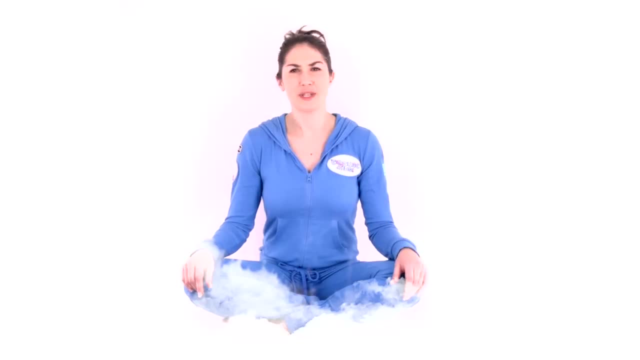 wants you to have a good time. He wants you to have a good time. He wants you to have a good time. All you do is hand them over. You take a moment to pack up all of your worries, every last one, and then you pass them over, putting them onto the bye-bye boat. 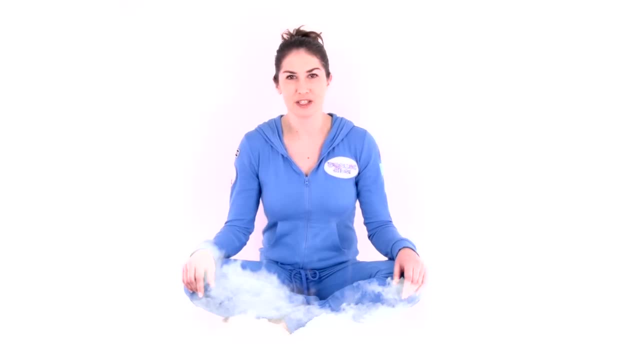 Next the kind old man asks for your anger. Again, he'd like to put you on the bye-bye boat. You gather your anger all up and you do just that. You put it onto the bye-bye boat, You agree? You say you'll go with me to the tie 창 and sail. You go with your order, saying How just it's so hard to breathe in it to他的. he on the bye-bye boat. You take a moment to pack up all of your worries, every last one, and then you pass them over, putting them onto the bye-bye boat. The good old man asks for your anger. You put it onto the bye-bye boat. 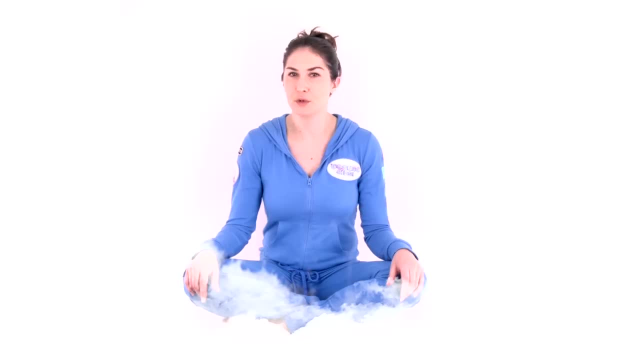 Finally, the kind old man asks for your fear. You make a special effort to collect all your fear, every last bit of it, And you hand it over, putting that on the bye-bye boat too. The old man looks and smiles at you. 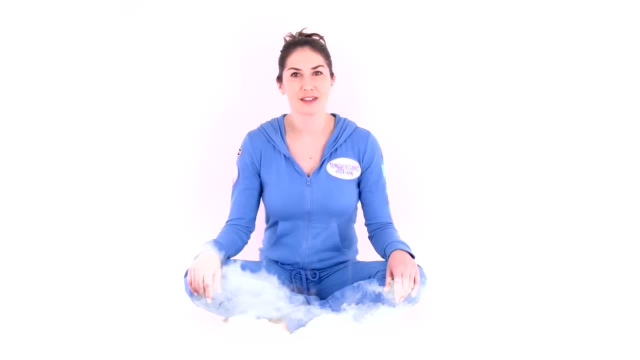 You smile back at him, enjoying the moment. You feel so good now. You feel light. You don't have any worries, anger or fear to carry anymore. You are free. The old man starts the engine. He raises his hand and gives us a little wave. 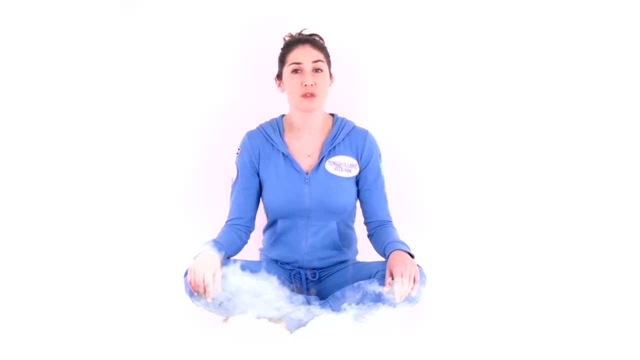 With those kind eyes and that warm smile, And he drives the bye-bye boat away. We lay back down And once again feel the warmth of the sun on our skin, The gentle rocking of the waves And the sounds of the ocean lulling us into peace. 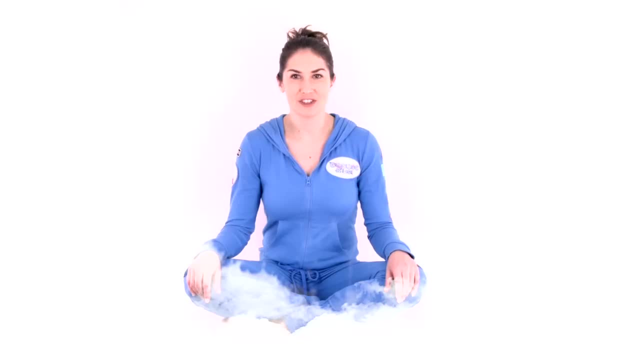 When we're ready, we head back to the beach, Our boat gliding gently over the water, Carrying us back to the sandy shore. We sit up tall and stretch. As we return, We turn to land, Opening our eyes to come back to where you began your meditation. 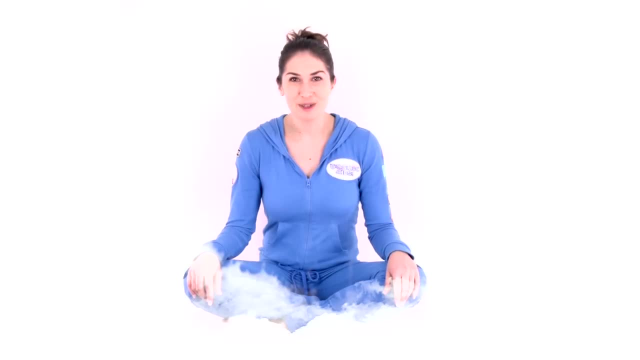 Wow, Well done you for taking this journey And for helping your body, mind and heart feel so much lighter By letting go of the worry, anger and fear. You can use the bye-bye boat whenever you need to. There's always a way to let go of the stuff that holds us back. 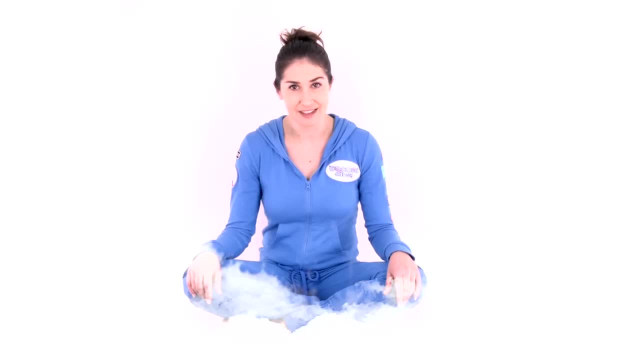 And usually that stuff is worry, anger and fear. Once we move these blocks out of our way, we are free And a whole load of possibility opens up. It's nice to know we can help ourselves get free like this. Your practice here in the Cosmic Kids Zen Den will always help you. 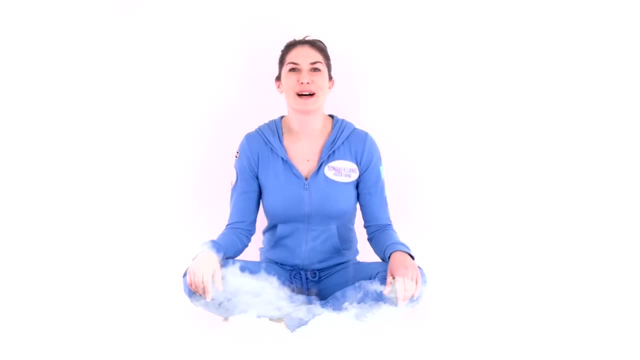 Keep it up And you'll soon become a true Cosmic Kids Zen Den master And you'll soon become a true Cosmic Kids Zen Den master And you'll soon become a true Cosmic Kids Zen Den master. Bye-bye, Bye-bye. 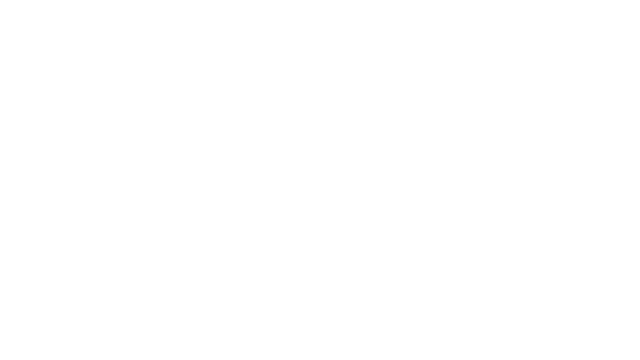 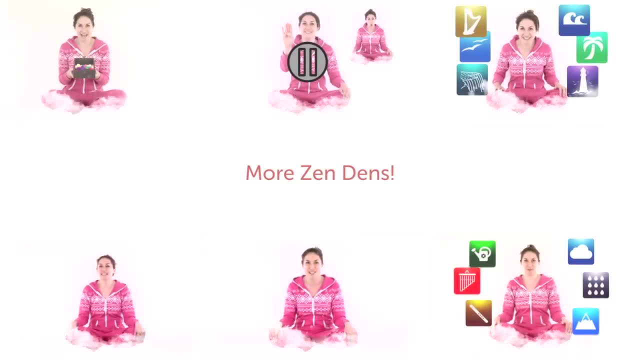 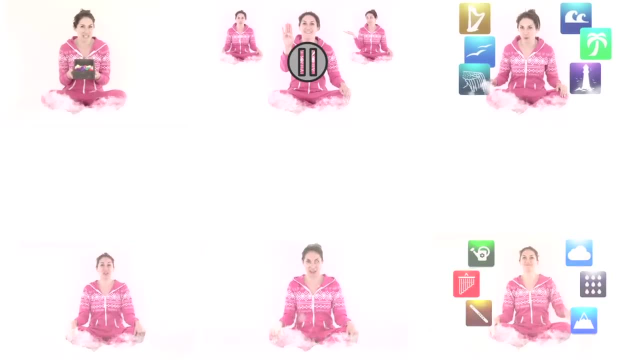 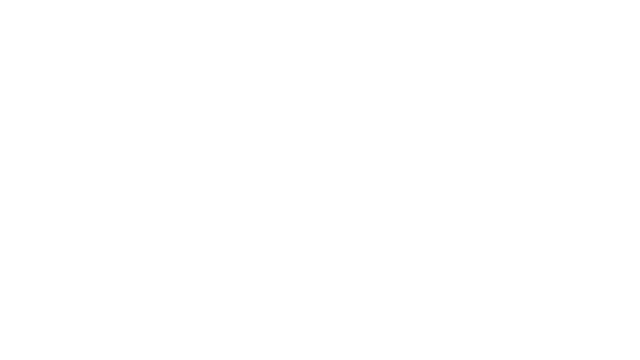